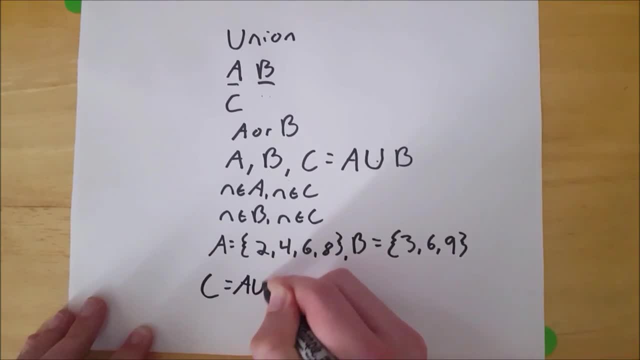 a set C that's equal to A union B. so the question is: what is that set going to equal? well, let's see, it will have 2, it will have 5 and 6, and then we're going to take another set B, which is equal to all. 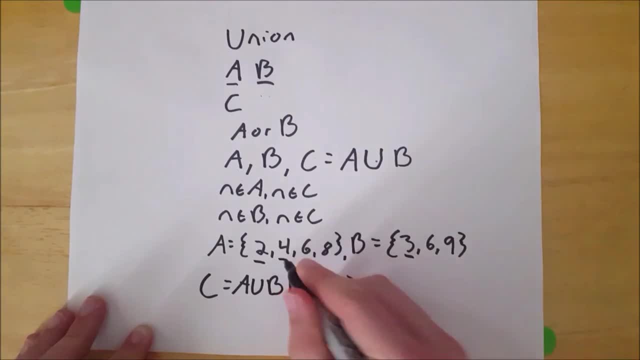 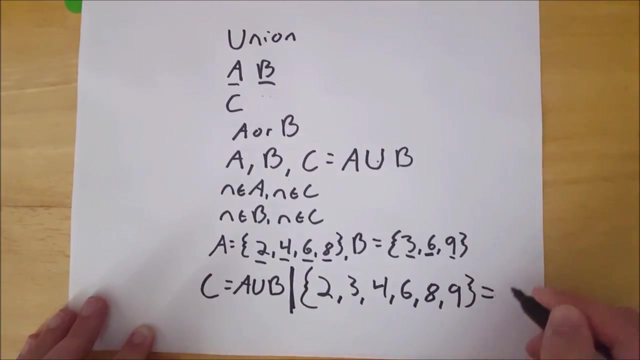 3, it will have 4, it will have 6, and remember that we only include distinct elements in a set, so you won't include six twice, even though it's in A and in B. A union B will also have 8 and it will have 9, and that's it. that is our set C. 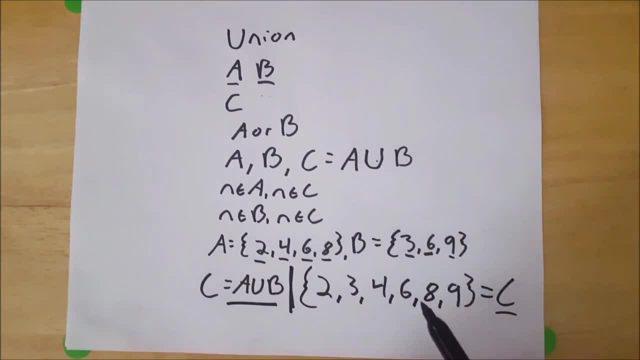 which is A union B, all the elements in A and all the elements in B and, by definition of a set, we do not include any repeats. so that's what a union is. I hope you found this video helpful. if you have any other questions about sets, unions or math, let me know in the 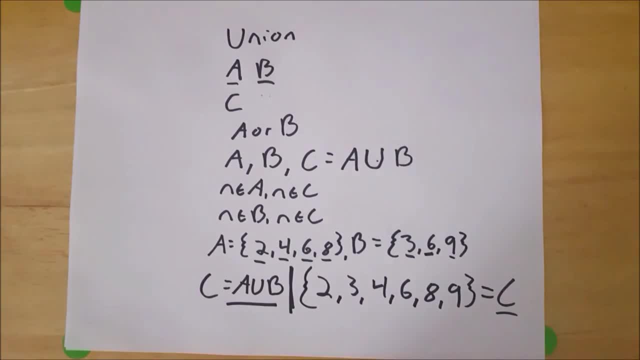 comments. I would be happy to address it, and have a lovely day. subscribe for more of these swankiest math videos on the internet.